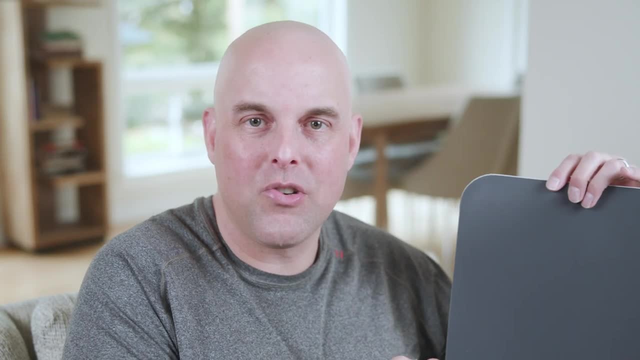 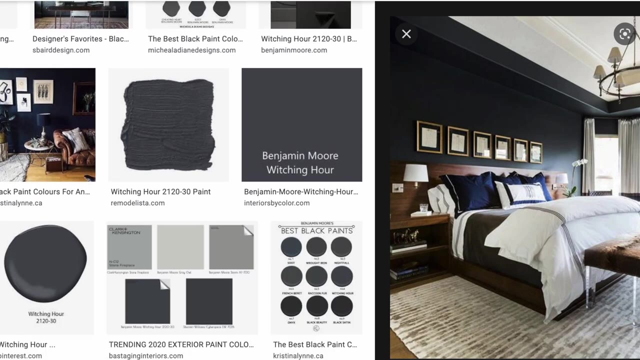 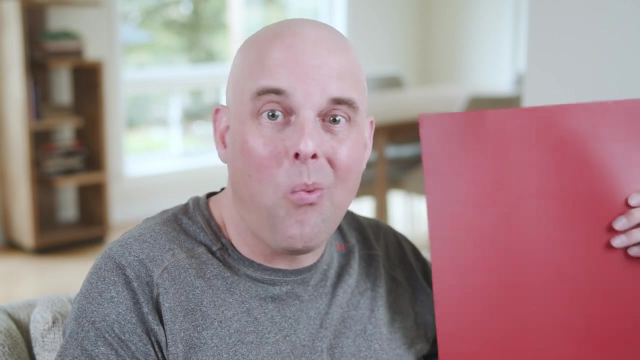 is a dark, rich charcoal gray. It's going to give you contrast. It pairs really well with Champagne, Gold, Off-Whites, Browns and Beiges, just to name a few. Now watch what happens when I compare it with Benjamin Moore Caliente, which is considered a dark red. Watch this When you compare Caliente. 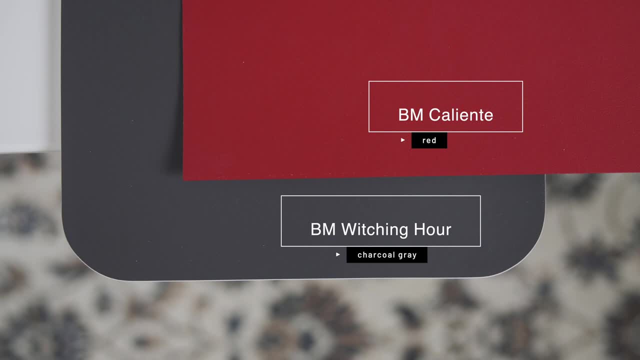 with Benjamin Moore Witching Hour. this is where you can see that dark, rich blue, and this is what I want you to know about this paint color. It's not a black, It's a dark, rich charcoal gray, and you'll definitely see more of that blue in real life, so be careful what you see online. 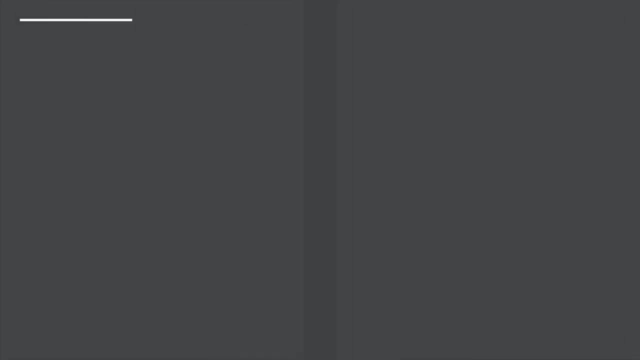 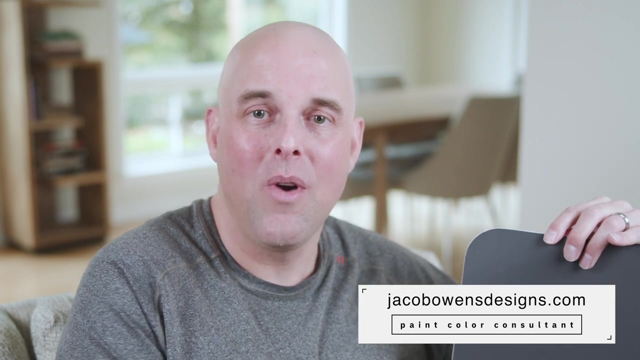 Benjamin Moore. Cheating Heart is a versatile charcoal gray. I did a recent paint color review about Cheating Heart. Go to my website. I'll tell you everything that you need to know about this beautiful paint color. You can use this for kitchen cabinets. 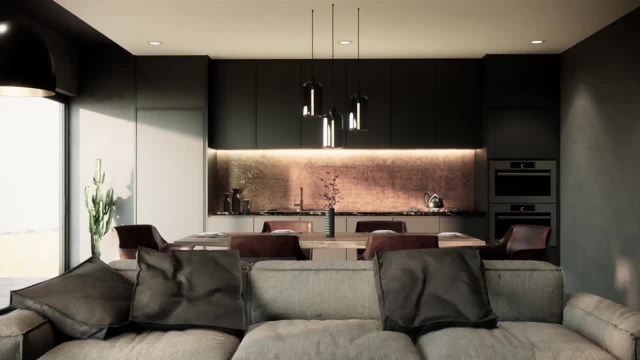 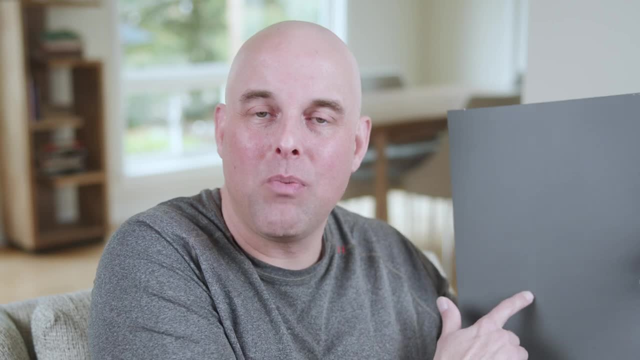 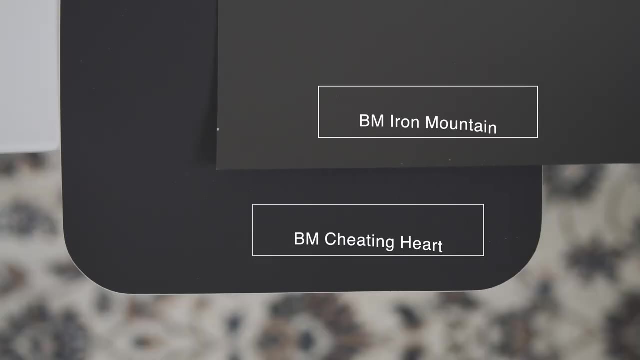 kitchen islands, built-in cabinets and exterior applications. To give you an idea just how dark Cheating Heart is, watch what happens when I compare this with Benjamin Moore Iron Mountain, which is considered a dark charcoal gray. Watch this When you compare Iron. 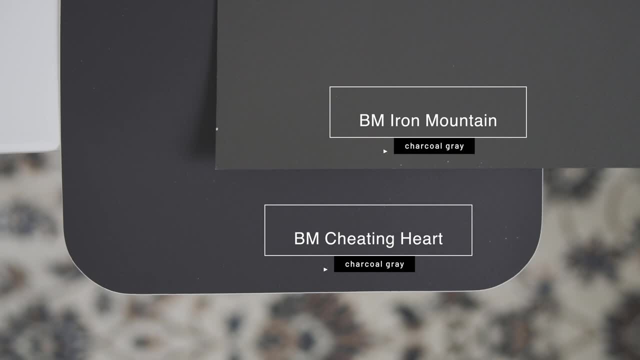 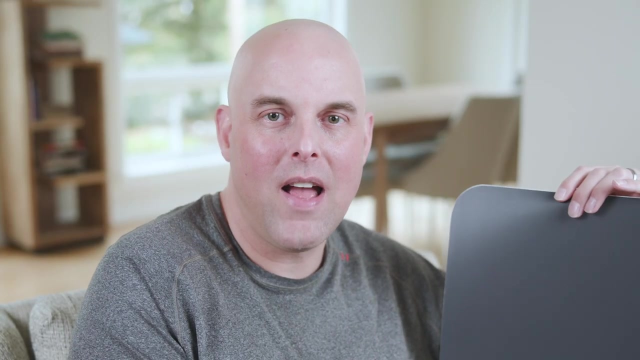 Mountain with Cheating Heart. this is where you can see that depth and contrast of Cheating Heart and if you look carefully, you can see that dark, rich blue in Cheating Heart. For those of you that are looking for a moody charcoal gray that's got depth and contrast. 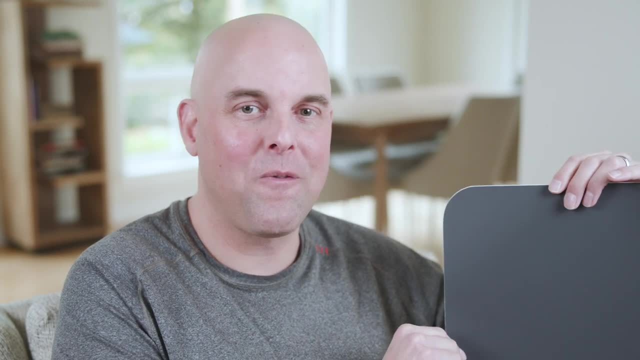 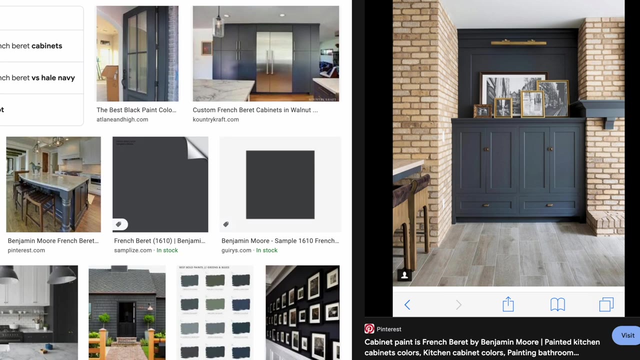 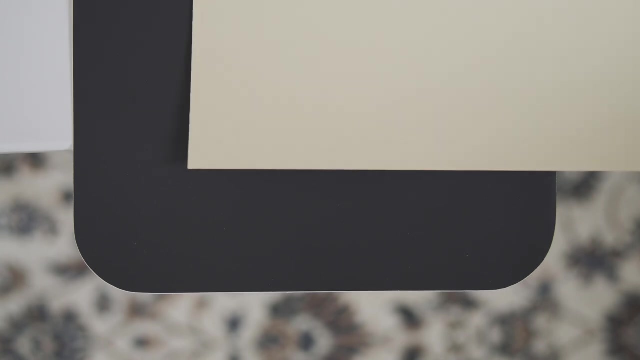 then French Bray could be just the perfect paint color for you. It pairs really well with browns, earthy paint colors and creams, just to name a few. Now watch what happens when I compare it to Benjamin Moore Western Flax, which is considered a yellow. Watch this When you compare Western. 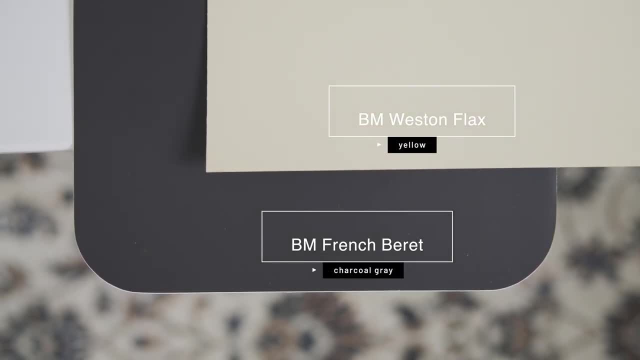 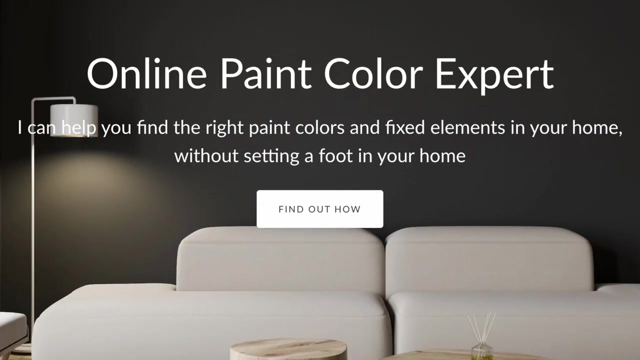 Flax with French Bray. this is where you can see that dark, rich, charcoal blue underneath French Bray. It's absolutely beautiful. For those of you that want to save time and get it right the first time, I highly encourage you to go to my website and check out my online packages. I can help you.